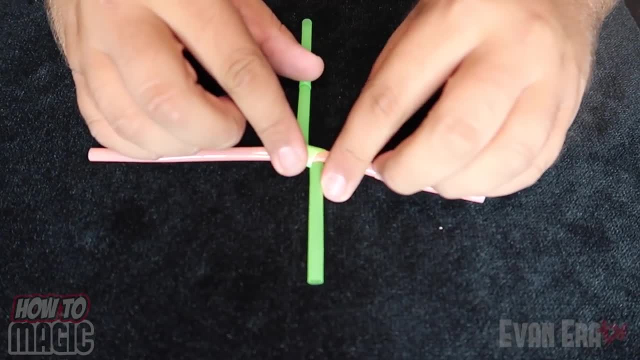 Okay, Here's the secret: It's going to go over the top of the other straw, go over around and down, just like that, wrapped around, just like this. so you have this cross. now the next step is to take this side of this straw, and it's going to go. 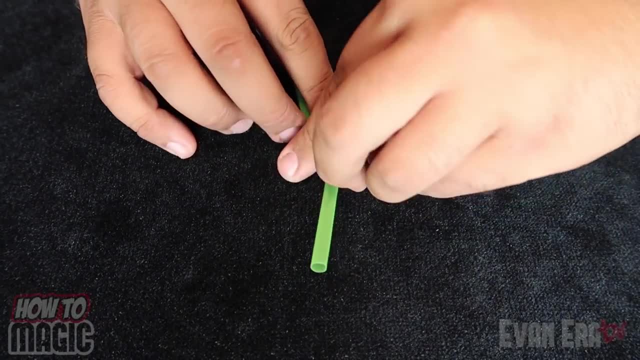 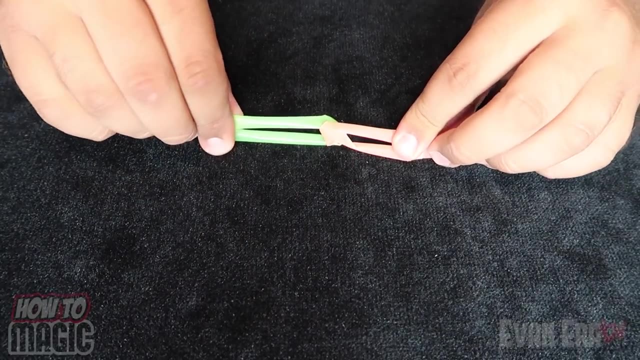 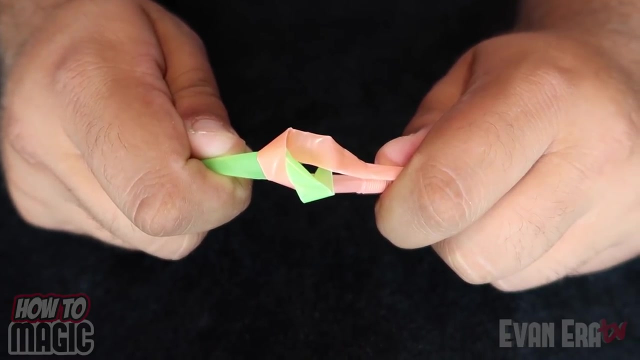 right there into this corner and it's going to wrap around like this and then one more time over, grab here and here, pull to make it look like they magically unlink. so once you have them in this position, they're not actually linked together, they just look like they are. so then you can do. 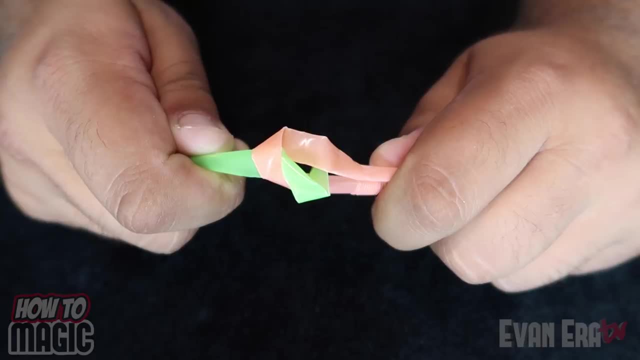 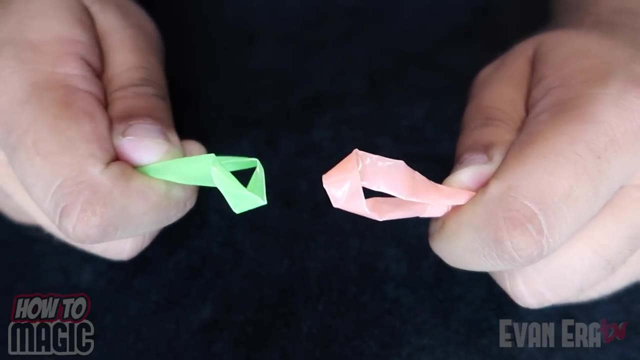 a little subtlety. you can blow on it, you can have your spectator rub it with their finger, you have them wrap their hand around it. then all you have to do to make them magically unlink is pull. they'll come apart and you can instantly unfold them and hand them out for examination. there's no cuts, no. 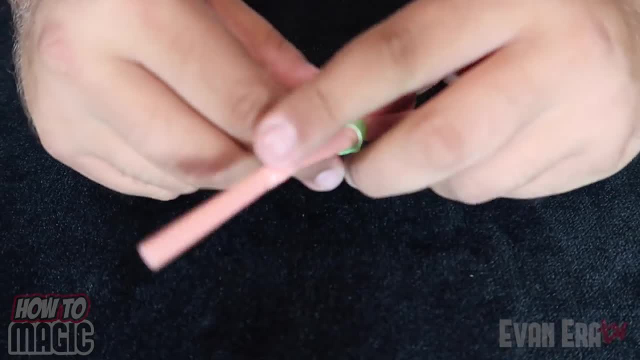 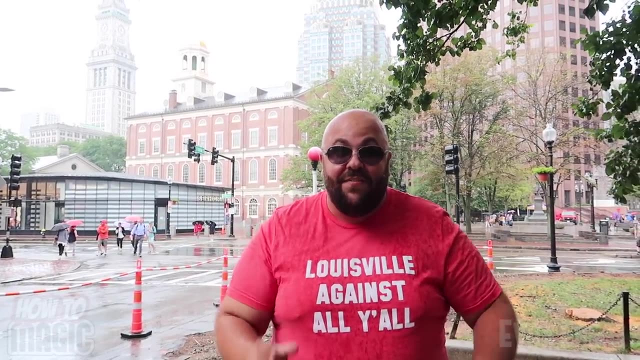 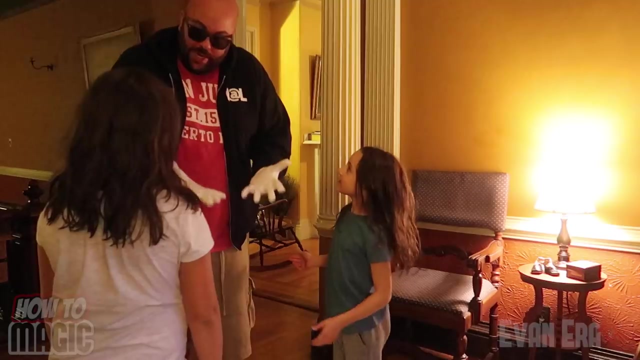 tears, nothing to find. straws just magically pass through each other, and that is how you do the magic linking straws. okay, this is an awesome magic trick. this is the growing glove. check it out, scarlet and ava. would you please assist me with this trick now? do you all know why magicians wear white gloves when they perform? 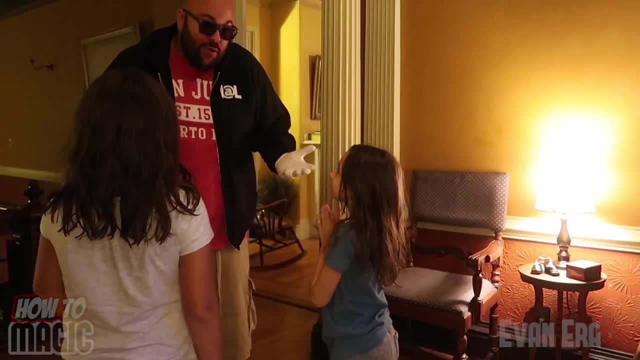 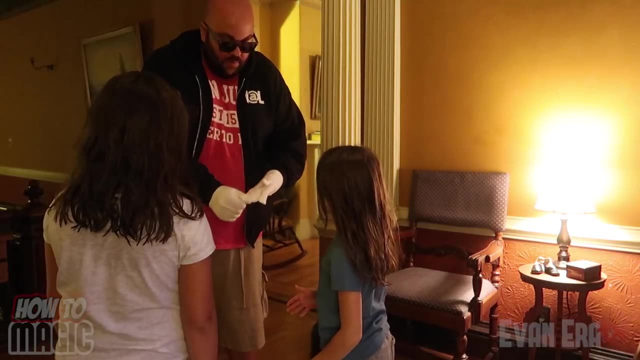 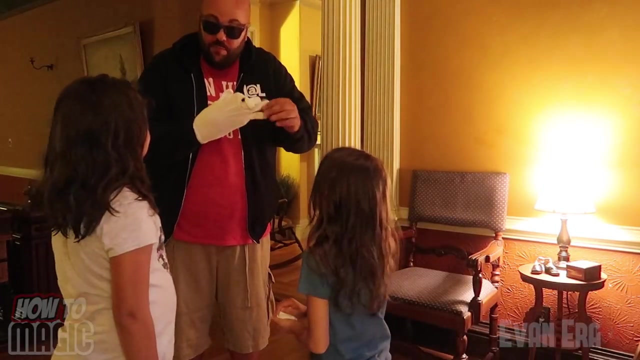 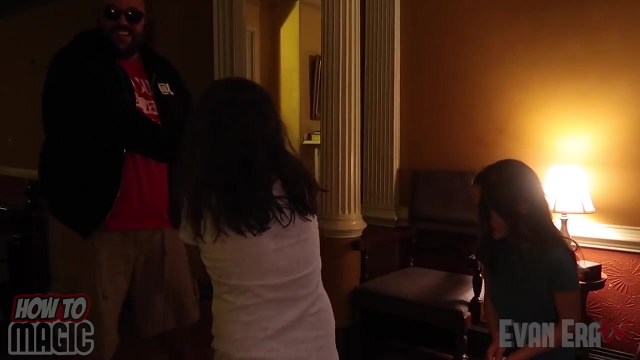 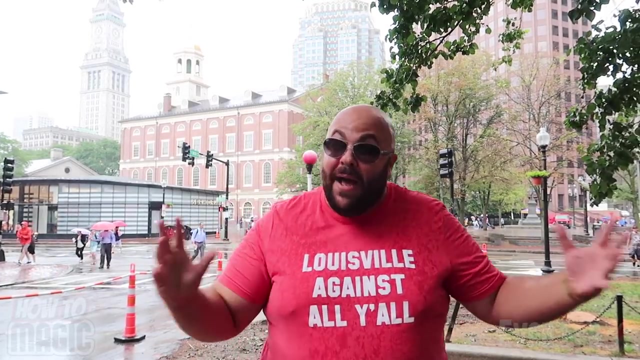 because it looks good. sure, i actually don't know. i thought you would know if you would scarlet, please remove my white glove. let's pull it right off. thank you. now, ava, would you please remove my right glove? eight, and then you do one trick after another, haha. 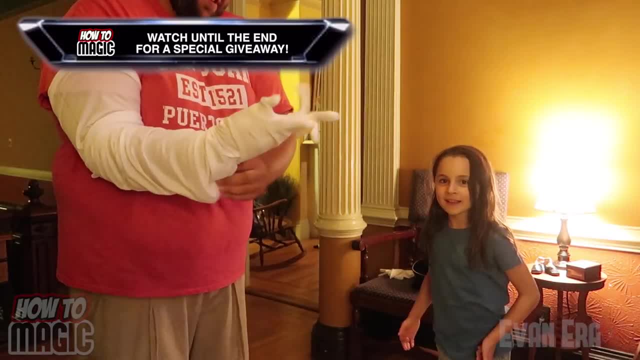 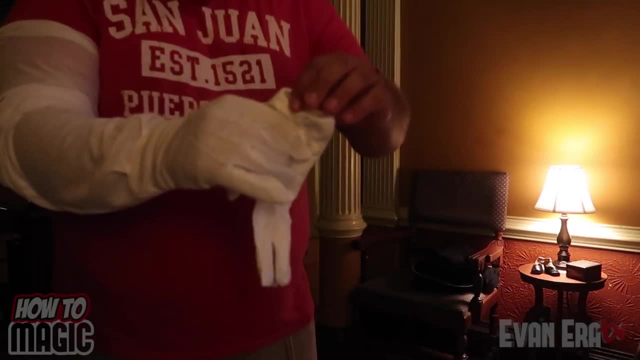 wow, i went sera through. hey, this is the secret behind this cool magic trick. this is the secret. all you do is take your super long glove and you put it up your sleeve. so you put your glove on and then you have your normal glove and that goes on the other hand. so you've got your long glove on this arm, normal glove goes over here on this hand, and then you put a jacket over top of it. 논. 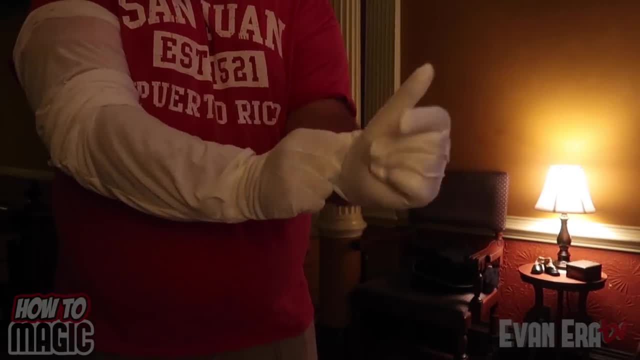 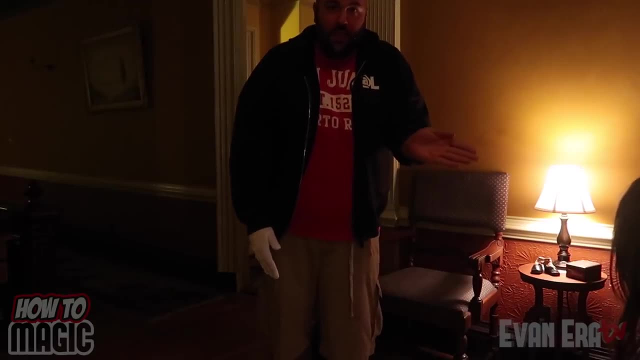 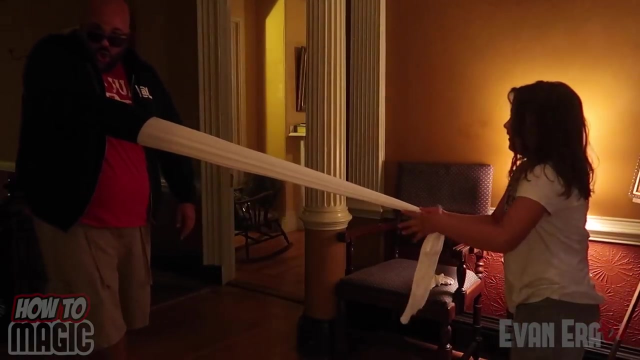 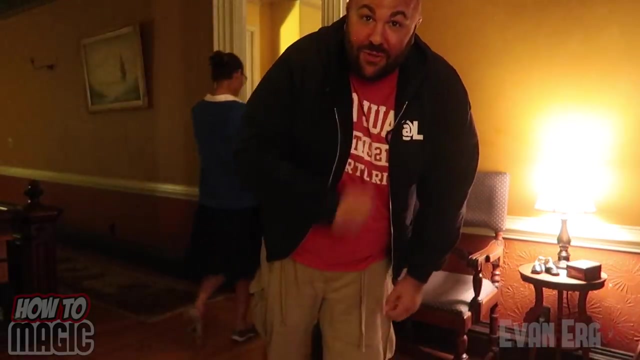 rainer and it looks like you're just wearing normal white magician's gloves. now you're completely ready to go, you can say: move my glove here. would you pull that off here, thank you very much. and just hold that on, just pull that off, and it's that easy, simple and fun trick that you can do. 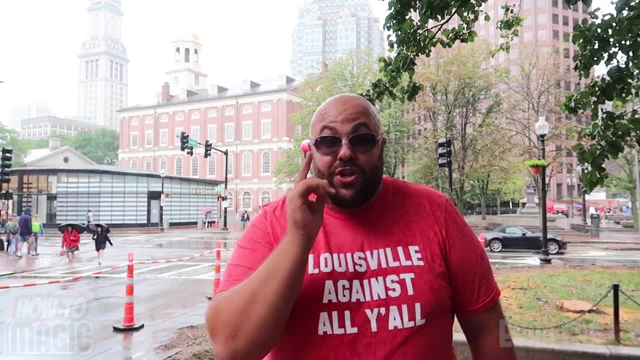 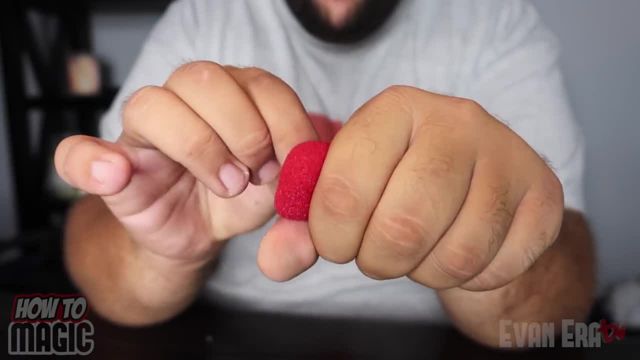 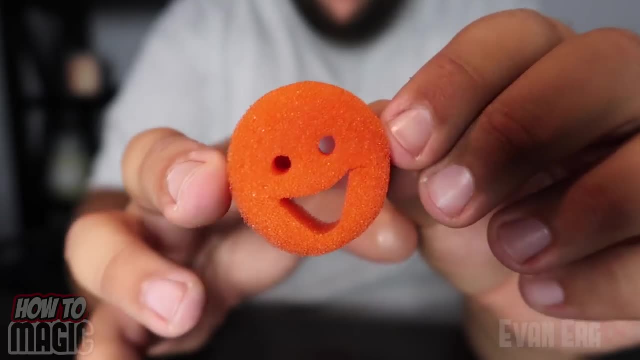 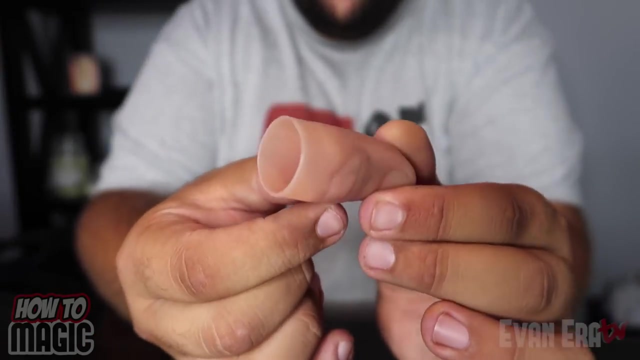 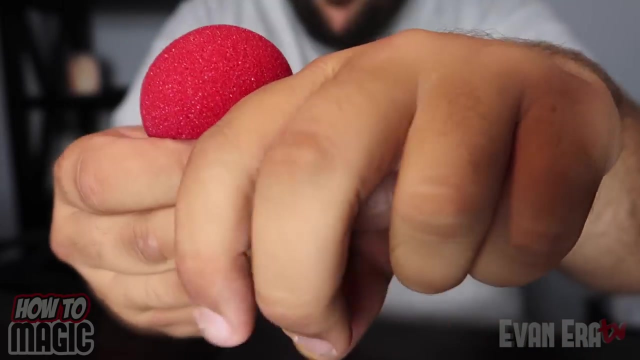 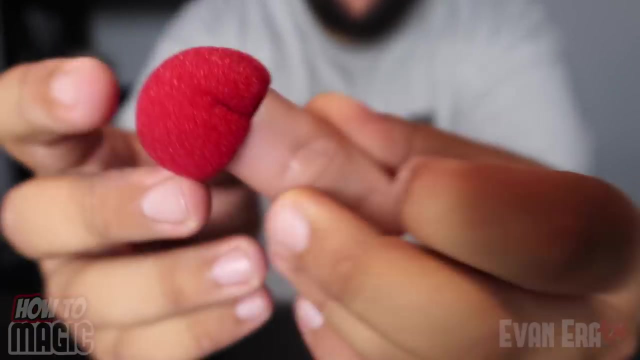 and that is how you do the magic growing glove. here's a really fun one that you can do at home. this is the spongebob to the smiley face. check it out. okay, here's the secret to the smiley face. check it out, so so so. 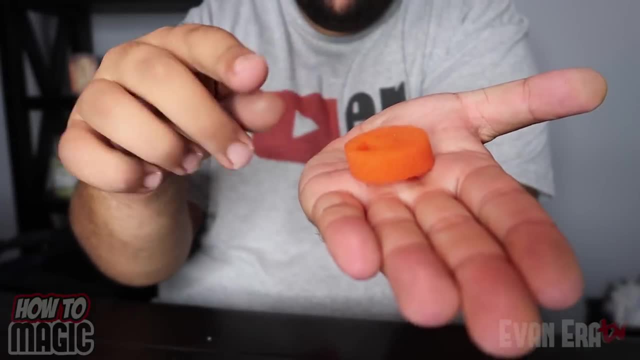 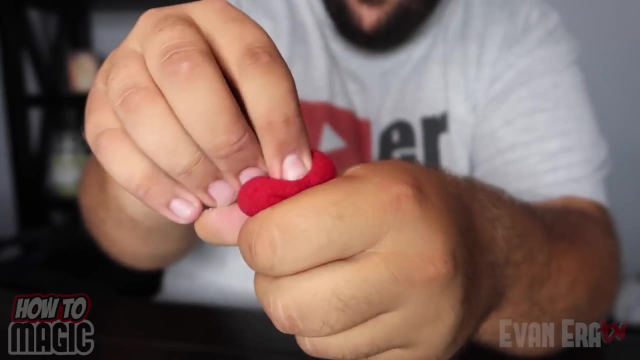 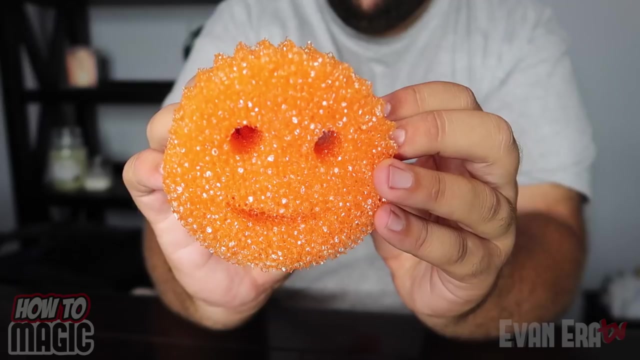 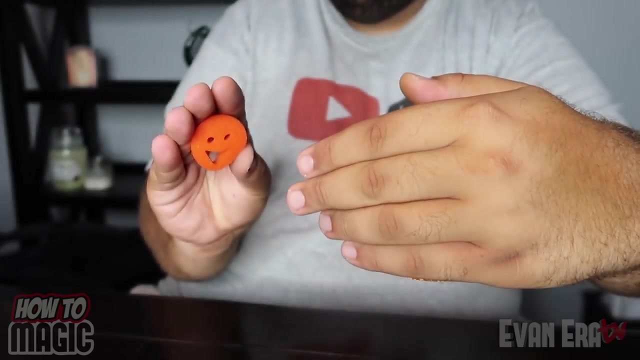 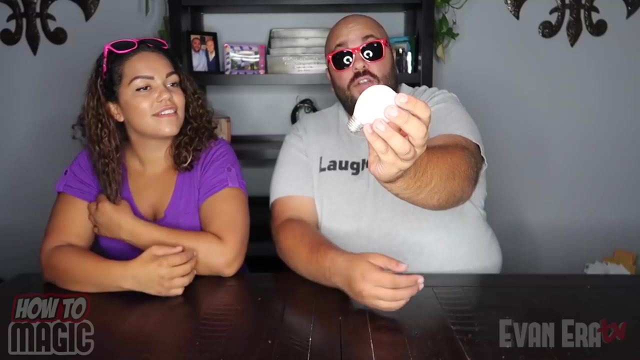 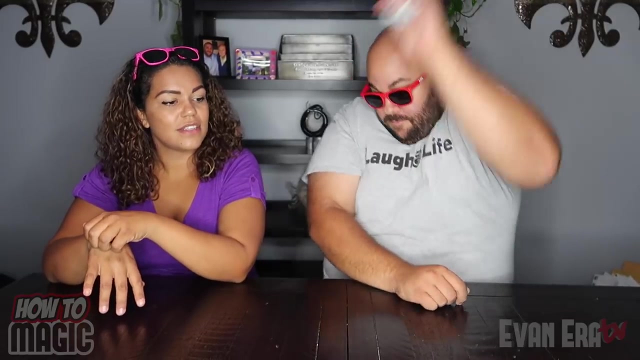 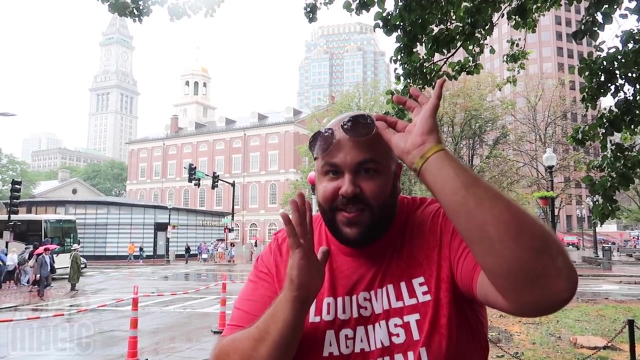 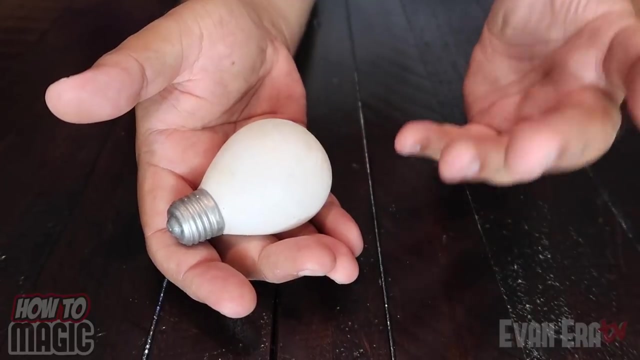 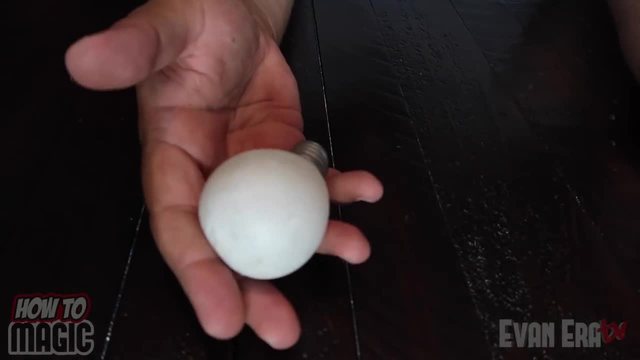 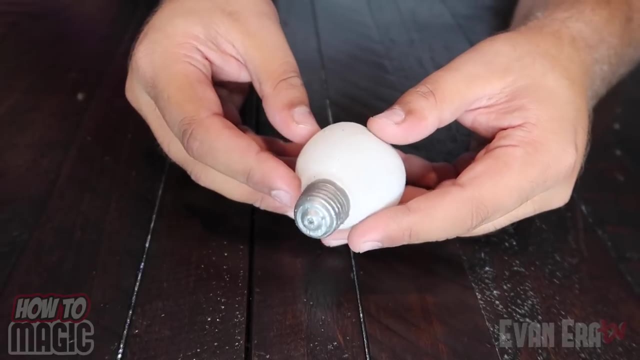 They're super squishy and kinda sticky, so if you throw it against the ground really hard it just sticks, just like that. Super cool, You can have this. show it off as a normal light bulb. You just don't want it to jiggle too much. 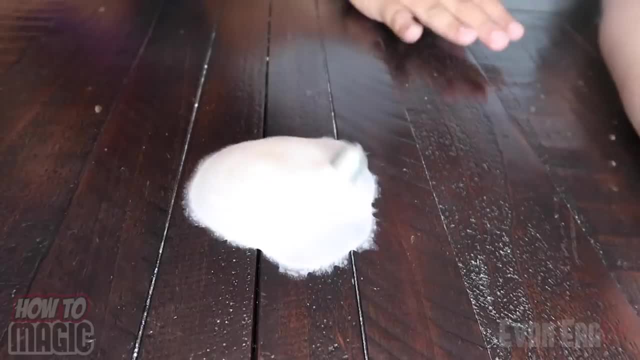 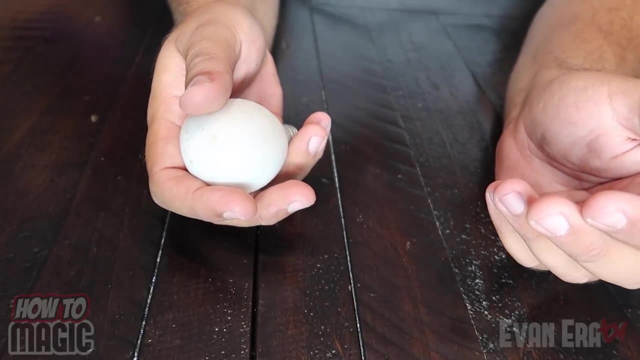 You can be holding it in your hand and say, watch, I'm gonna take this light bulb. you can throw it on the ground at your spectator's feet. They'll totally freak out, thinking the light bulb's gonna shatter. Or you're gonna say, watch, take my light bulb. 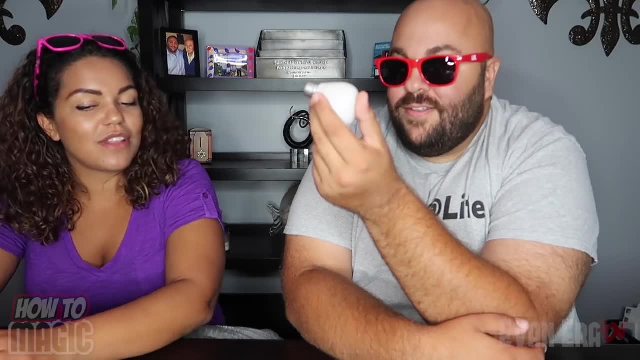 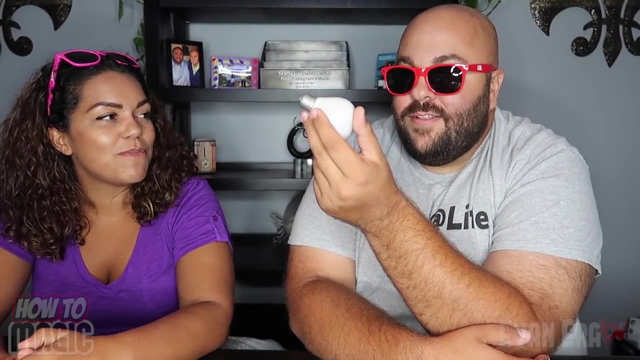 watch the light bulb, Say your light went out, and then toss it down to your mom. or your mom asks for a light bulb. Oh, you have somebody ask for a light bulb, throw it to them. Yeah, just have it on your hand. 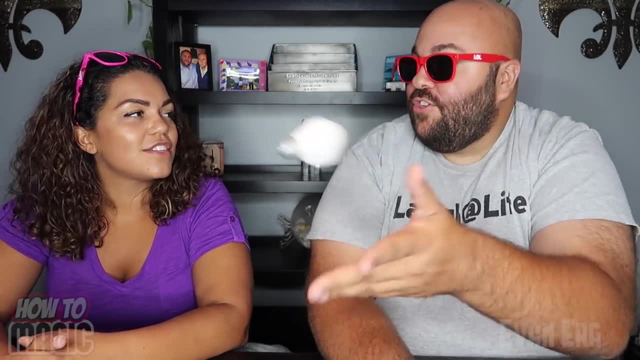 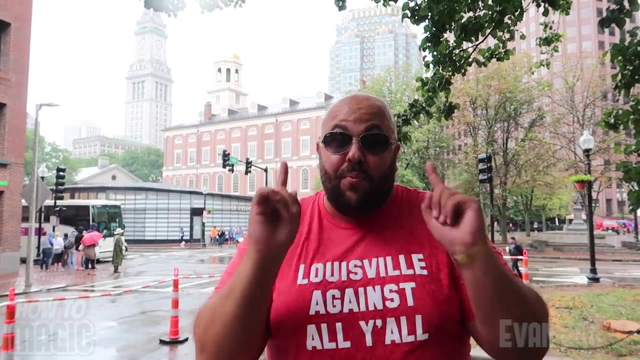 And just toss it to them and then they're like: ah, Oh, that's funny, I hear a catch. Yeah, like that, And that is how you do the magic light bulb trick. Okay, for this one you're gonna take two breath mints. 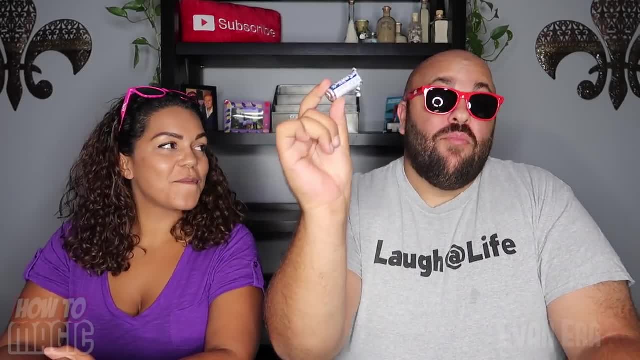 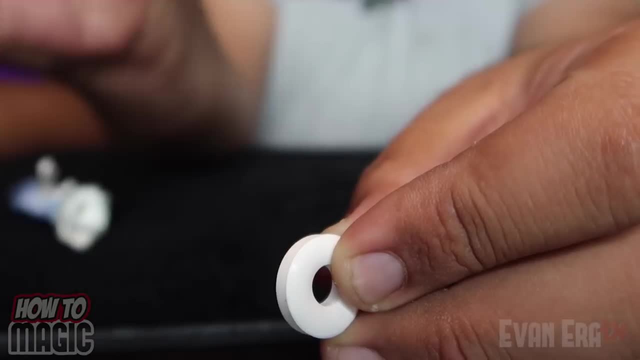 and blow someone's mind. Check it out. Okay, this is a cool one using breath mints. You're gonna take two mints in this case. I'm gonna use these two right here: One, two, three. What? 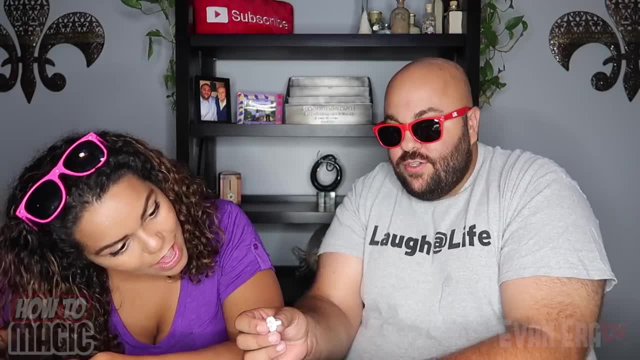 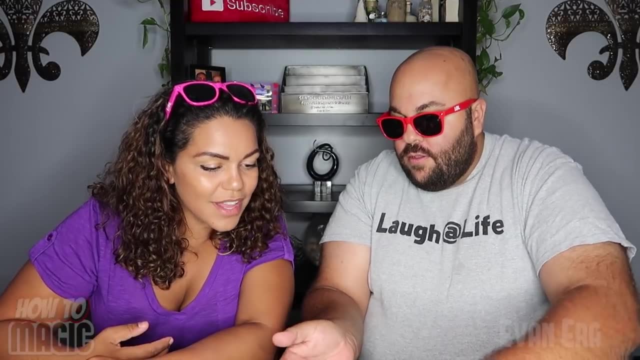 What See them link together? Yes, All right, watch One, two, three. No, And they're both home. Are you serious How? I'll teach you the secret right now. Okay, here's the secret. Okay, the secret behind this trick is: 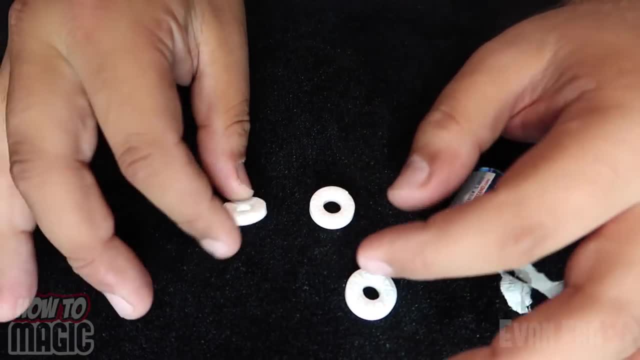 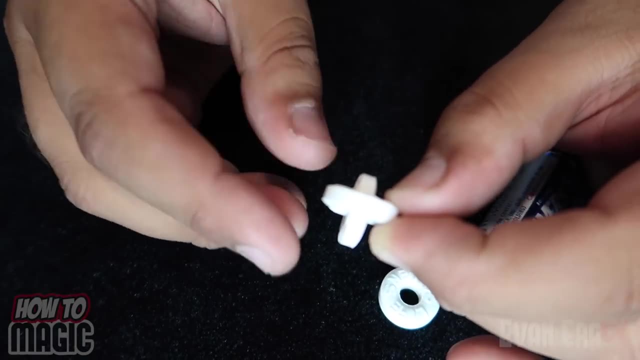 these are not real breath mints. They're rubber- This one's rubber and this one's rubber- and it has a small cut in the mint so that it can pop right on there just like that. This is a real mint. These are fake ones. 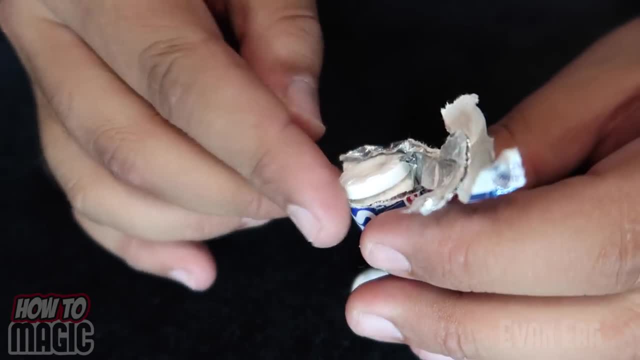 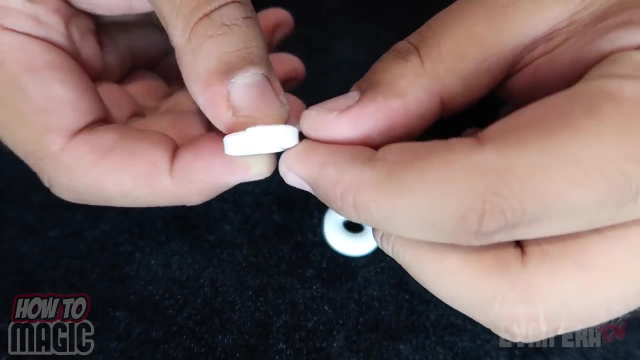 Really hard to tell the difference. You can start the trick by having your fake ones inside your roll of breath mints, Take them out and say: watch, Take the two mints. You wanna position it so that this little cut that is lined up right above. 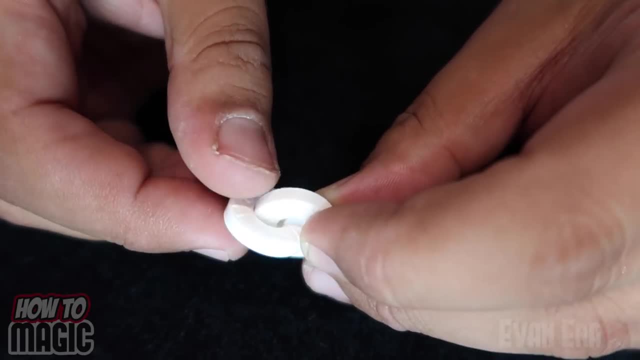 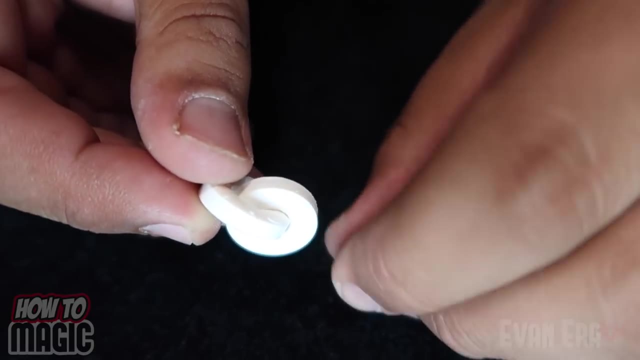 where it's gonna go through the mint, just like that, so that when you push down, two halves separate and it's able to go right there through that hole, and then you can spin this mint around and say, look, they've magically linked together, like that. and then, just as quickly as they've linked together, 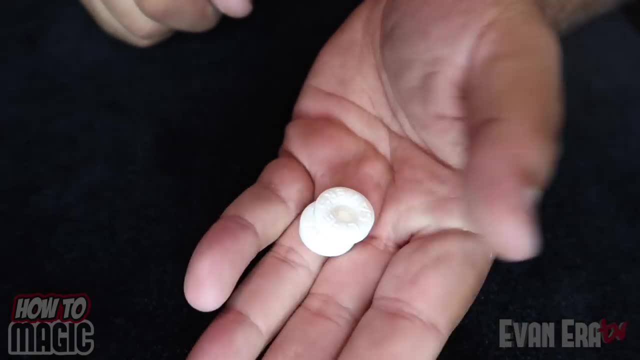 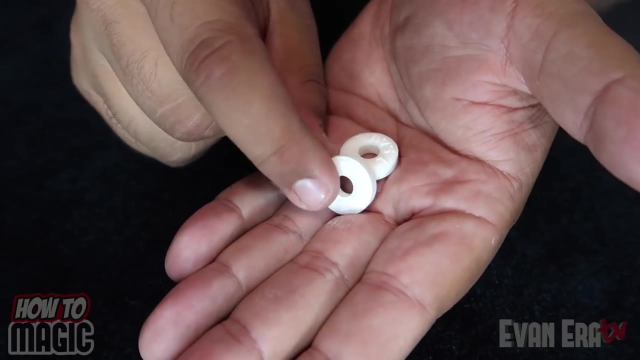 you can magically pull them apart. You can then swap these out with real mints and hand them out to your spectators for examination, and they will be absolutely baffled. It's a simple trick that has an awesome effect. Awesome secret. Stay tuned to the end of the video for a special giveaway. 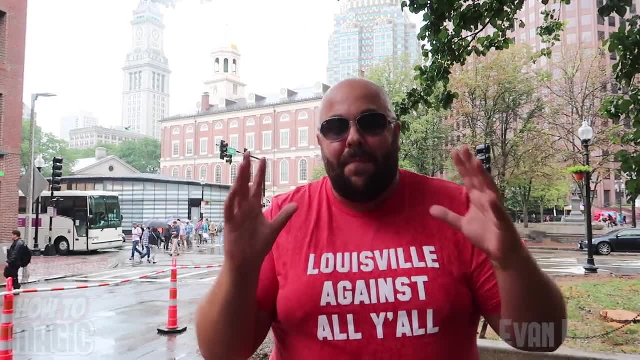 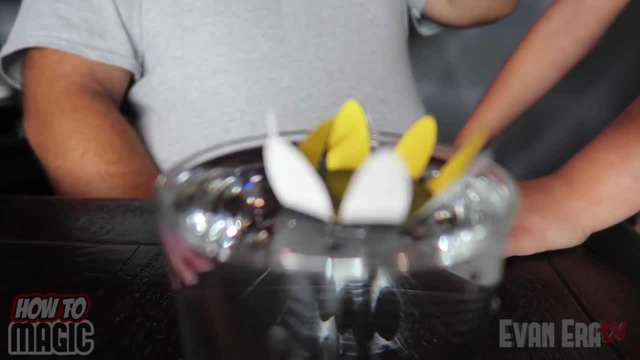 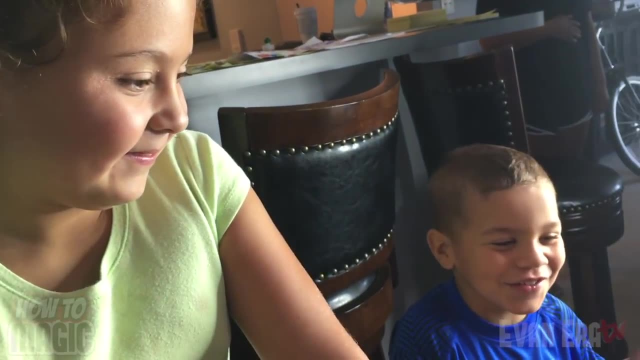 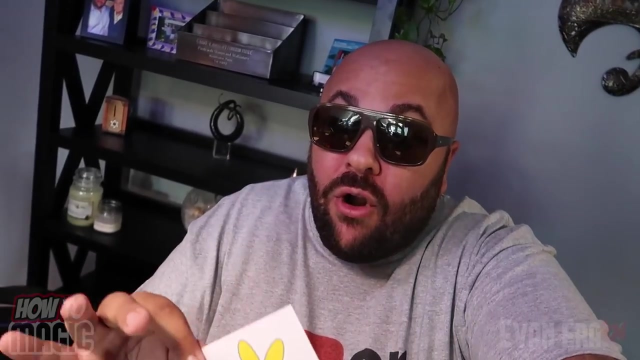 And that is how you do the magic linking mints. Okay, this one is the blooming paper flower. Check it out. The secret to this one is a lot more simple than you might think. Take a look, All right. so really simple here. 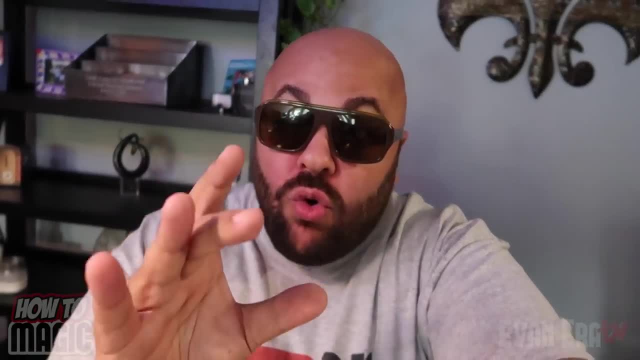 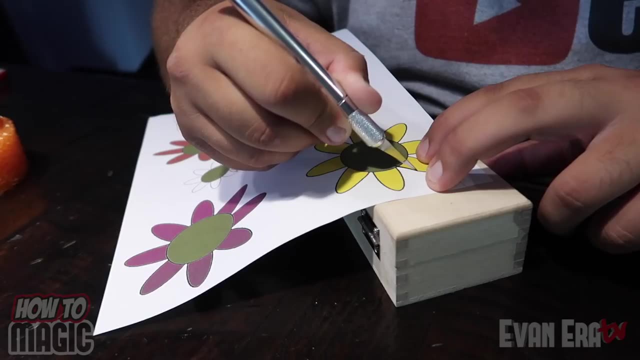 All you're gonna do is print out one of these pieces of paper. You can find this online by just going to Google and typing in blooming paper flower. It'll pull up this image. You can print it out on your computer. Then all you do is cut out your flower.